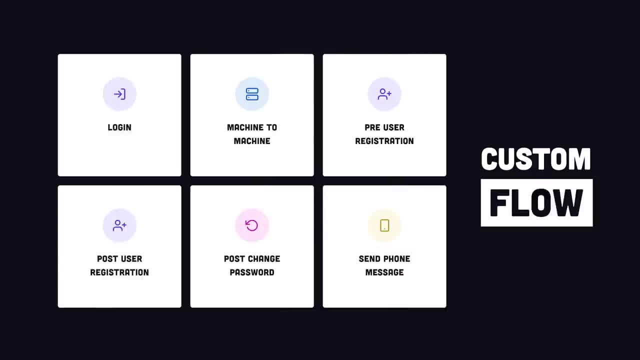 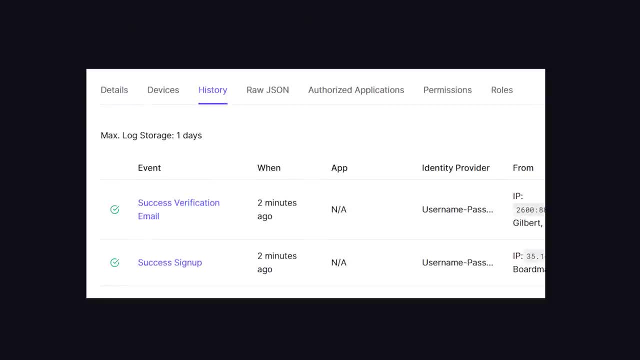 methods out of the box and allows you to customize the flow with a click of a button. After signup, each user is assigned a unique ID and the record can be managed from the dashboard. You might view their login history or devices, or maybe you want to block a malicious user. 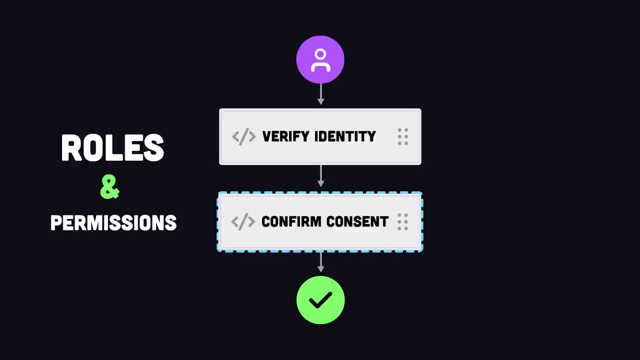 You can also define custom authorization logs, and you can also define custom authorization logs in the form of roles and permissions. You can then read this data from a front-end or back-end environment, with an SDK for virtually every runtime and a REST API for everything else. 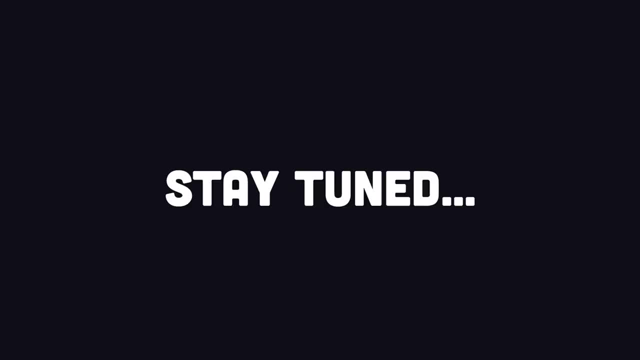 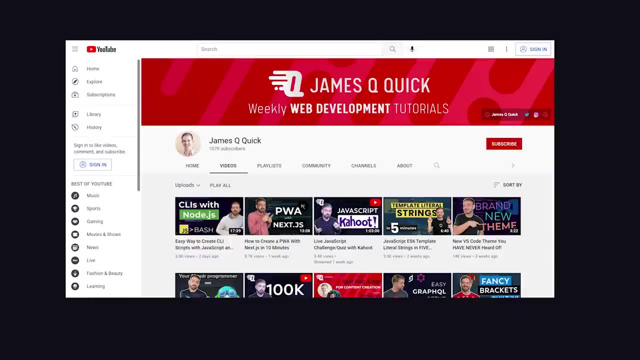 This has been Auth0 in 100 seconds, but stay tuned because I've invited a friend of mine, James Q Quick, to take us beyond 100 seconds to integrate Auth0 in a Nextjs app. He's a developer advocate at Auth0, and also has an awesome YouTube channel that you should definitely. 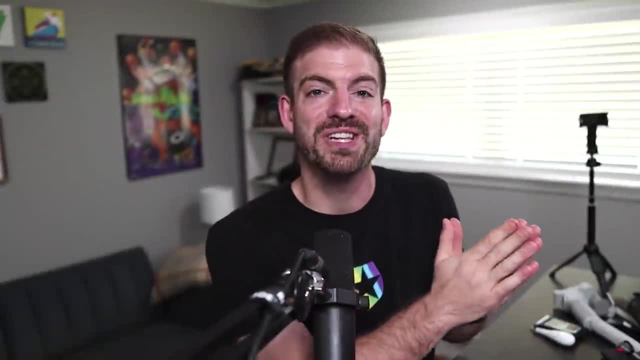 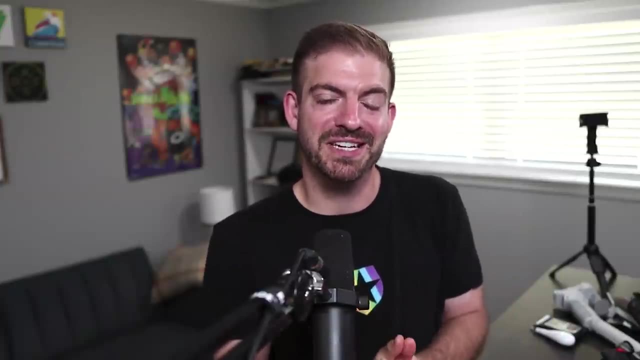 subscribe to. Hi everyone, my name is James and I'm here to take you beyond 100 seconds in your journey to learning more about Auth0. So let's go ahead and see how to set up Auth0 inside of a Nextjs application in less than 10 minutes. All right, so the first thing you'll want to do is 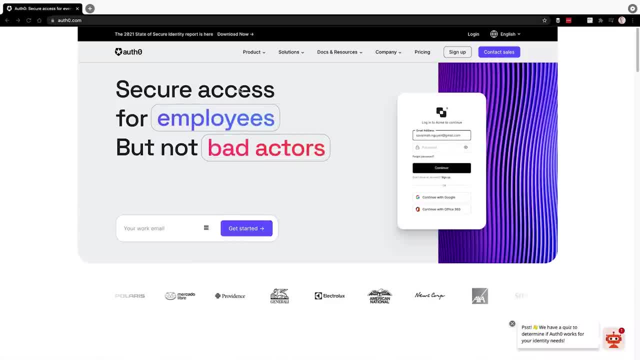 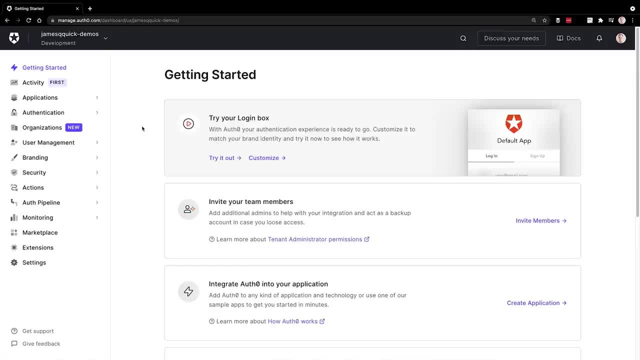 sign up for a free account in Auth0. You'll have a link that you can sign up with in the description below. So I'm going to go ahead and log in and then we'll get started creating our application. All right, now that I'm logged into Auth0, I'm here on the Auth0 dashboard. Now Auth0 has what? 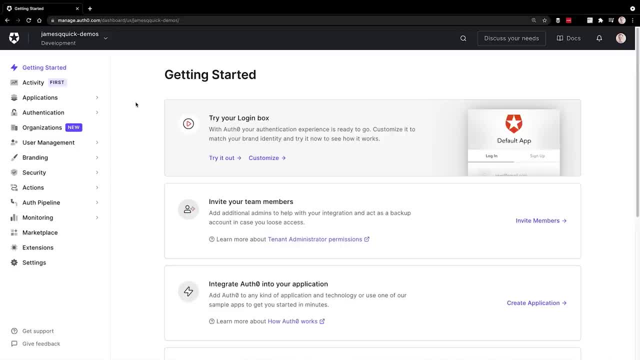 are called tenants and you'll need to create a tenant to get started. A tenant is basically a grouping of your applications, So in this case I'm inside of my James Kukwick demos tenant. From there I can go into applications. 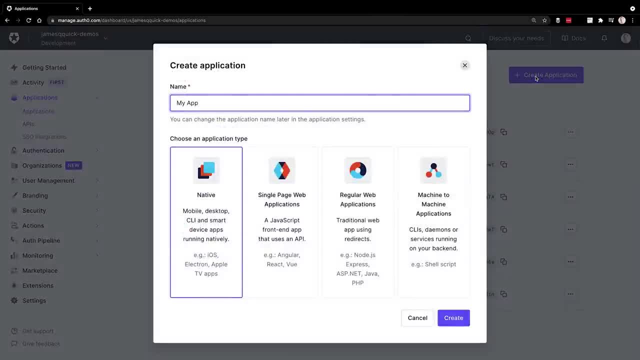 and I can create a new application. Now, when we try to create a new application, we're going to have a couple of different types. What we're going to choose is a regular web application. What this means is we're able to take advantage of the server side aspect of Nextjs, And so, in this case, 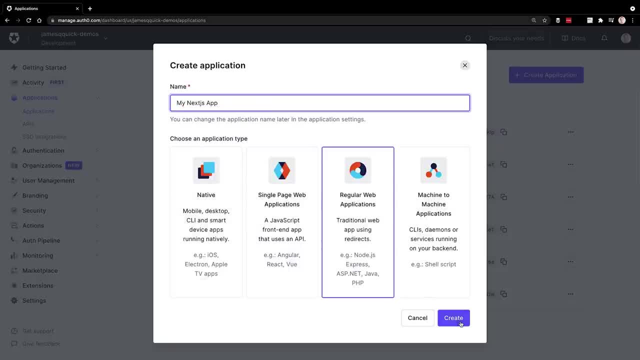 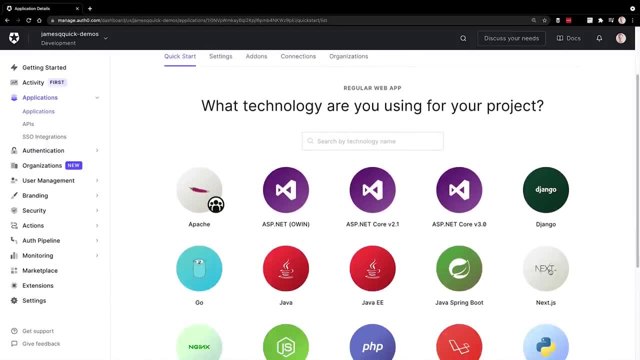 we'll create a regular web application, So I'll call this my Nextjs app- And then, after this is created, under the quick start, there is some starter code that we can use for a bunch of different platforms. So if you're not familiar with React, you're going to want to go ahead and 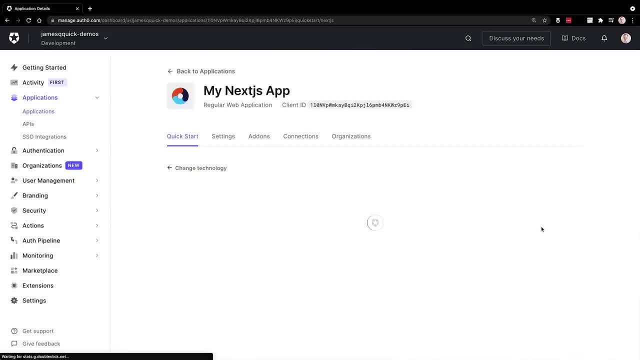 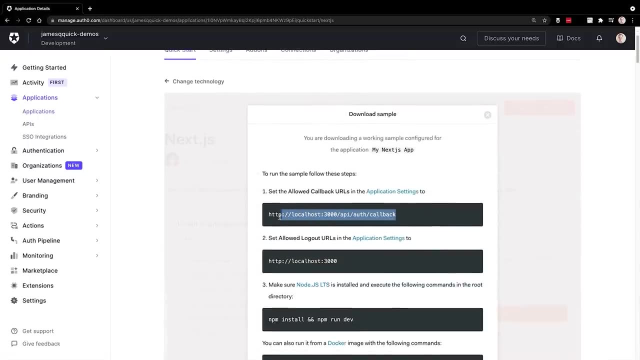 react to Nextjs. You can check out all the different platforms and frameworks that we have available to you to get started, But I'm going to choose Nextjs And I'm going to download this sample project And it says there's a couple of different settings that will need to update. 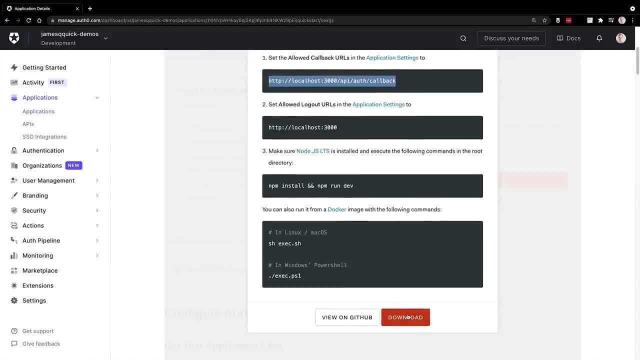 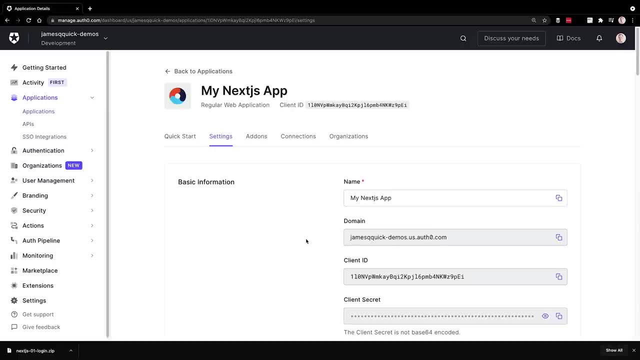 inside of the Auth0 dashboard as we go through this. So let's go ahead and download this repository. With that downloaded, let's go back into our settings And I'll show you a couple of things we need to pay attention to. When we open that source code, we'll need to know: 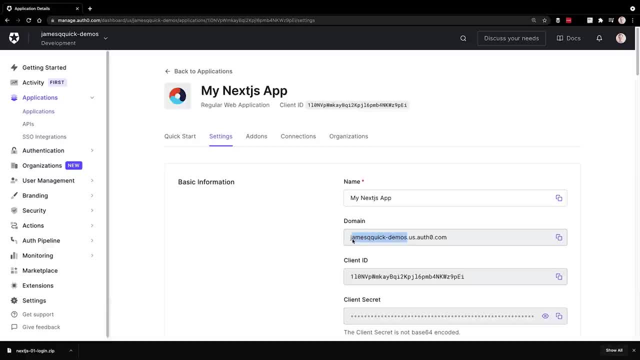 our domain and our client ID. The domain is our tenant, and then dot and then our geography here in usall0.com, And then the client ID is a unique identifier for this application. So one thing we need to do is scroll on down. 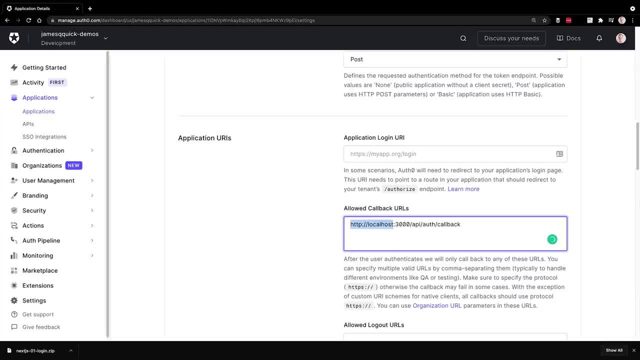 and update our callback URLs, And what this is is the acceptable URLs that All Zero can call back to after authentication happens. So we redirect the user to All Zero, they authenticate and they redirect the user back to this URL. Now this is gonna be an API endpoint. 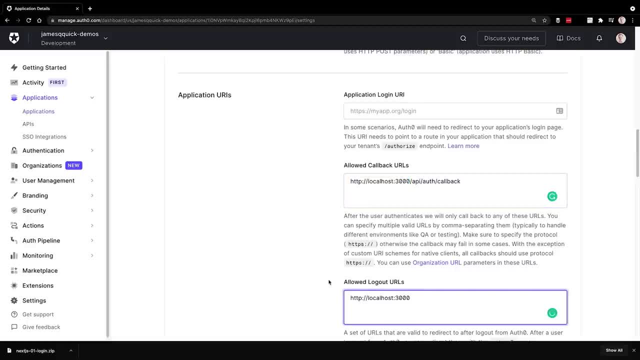 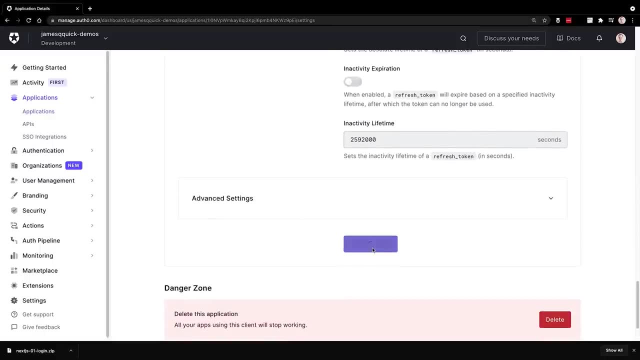 inside of our Nextjs application And then for our allowed logout URLs we'll just have localhost 3000.. So I'm gonna scroll all the way to the bottom, make sure to save these settings, and then I'm gonna open up this sample code. 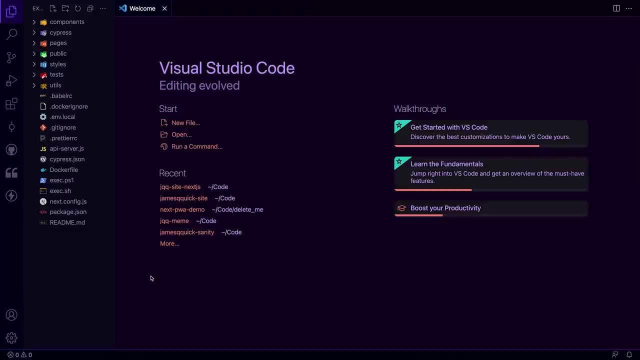 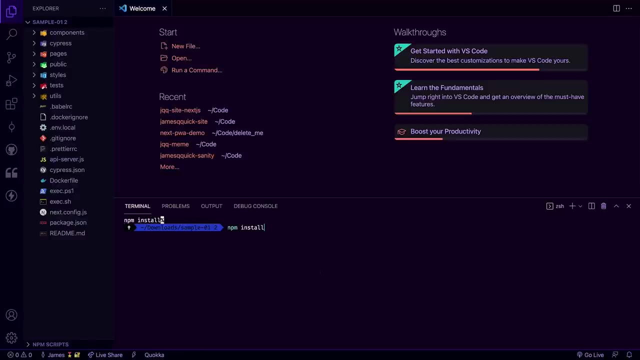 the starter code inside of VS Code. Okay, I've got that sample code downloaded and opened inside of VS Code, So the first thing I'm gonna do is run the npm install command, which will go and install all of our necessary packages. Now, as that is installing, 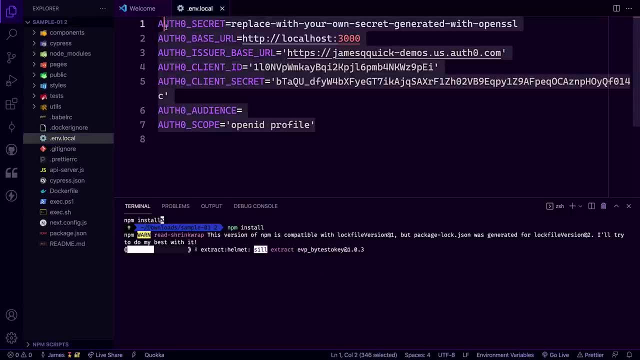 notice. we have a envlocal file and inside of this file we have configured a secret here where we need to replace this with some sort of random secret which is used to sign cookies. We could more intelligently create this, but for now we can just add in a random string. 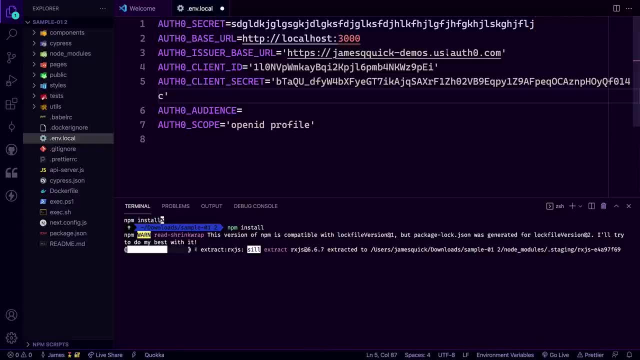 Then we have our base URL, which is the localhost 3000, the issuer base URL, which is that domain that we just looked at, the client ID, which is already populated in here, and then also the client secret. Now, because this has a server side aspect in Nextjs. 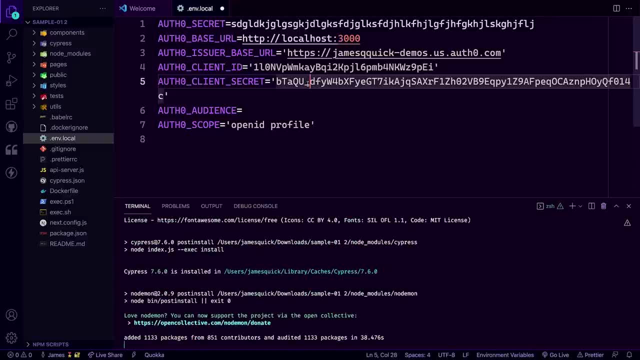 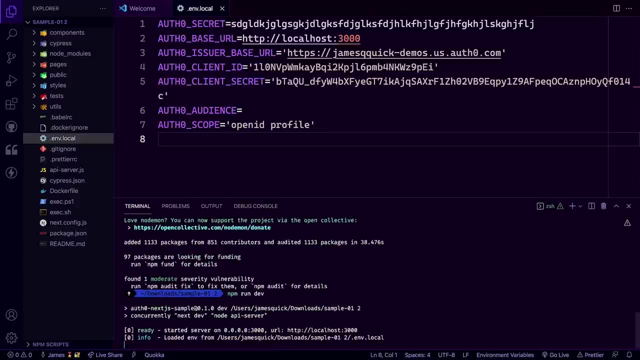 we're able to keep a secret, and in this case we can keep this client secret safely inside of our project. All right, with all of that in place, I'm gonna run the npm run dev command and this will start up our dev server. 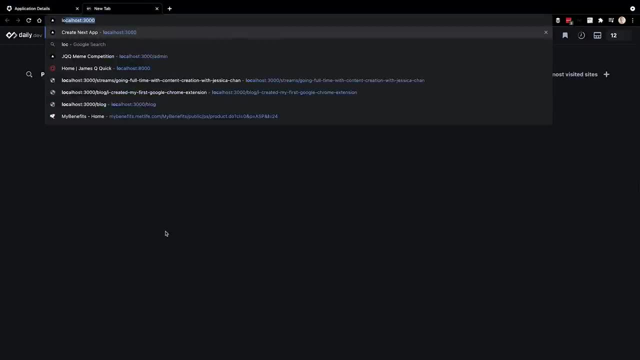 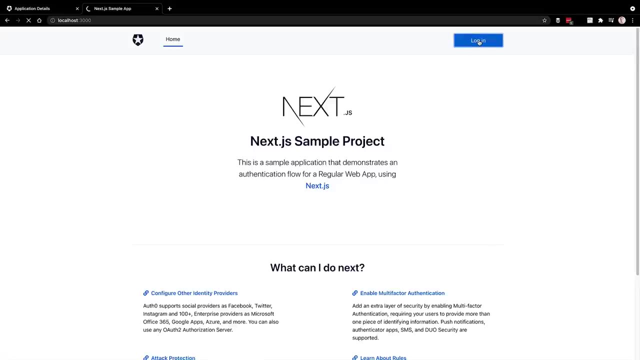 And so, after it is up and running, we can open a new tab to localhost 3000.. And once this opens up, notice we'll have this login button here where we can go ahead and log in. This will do the redirect over to Auth0.. 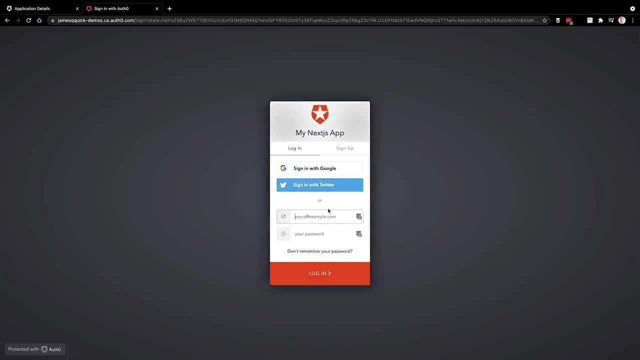 I've got a Twitter option configured here, but by default you'll have sign in with Google available to, and then you'll have the ability to log in with email and password. So if this is your first time, you'll have to go through the signup section. 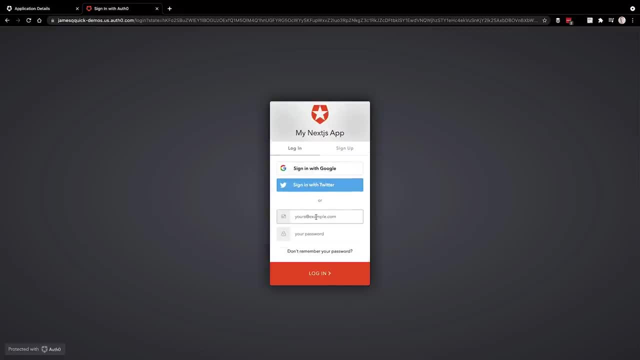 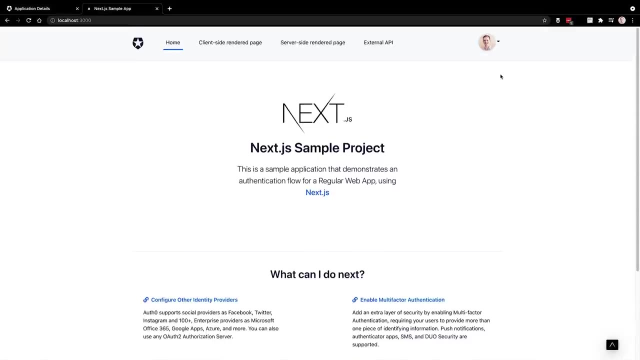 for your email and password, or you can choose the Google provider. In this case, I'm gonna log in with my email and password. All right, after I finished that login process, notice I've got my profile picture up here, and then if I go to the profile page, 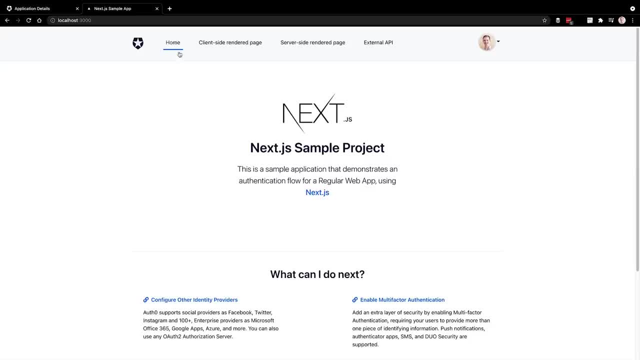 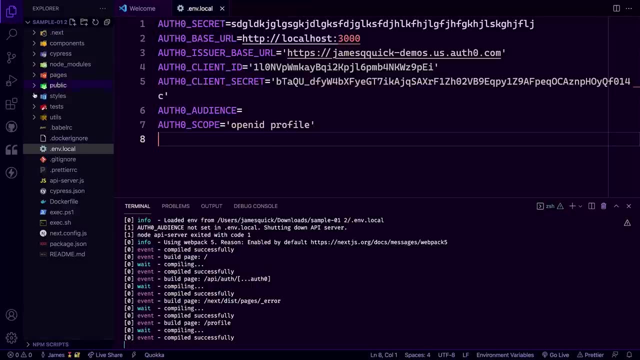 I can see a little bit of information about myself as a user, So you might be wondering: how much code did it take to implement all this? Well, I wanna show you how cool and easy it is to set up Auth0 inside of a Nextjs. 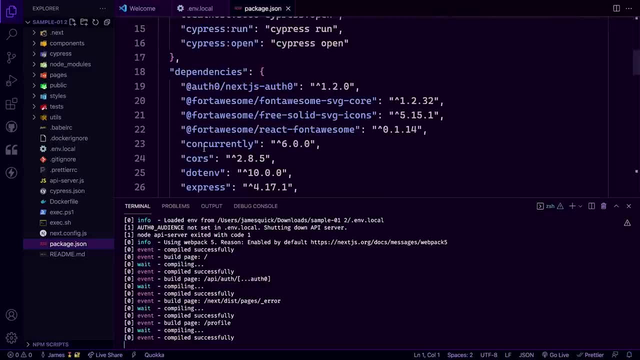 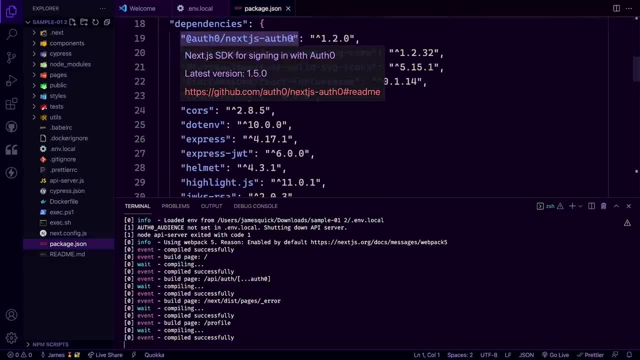 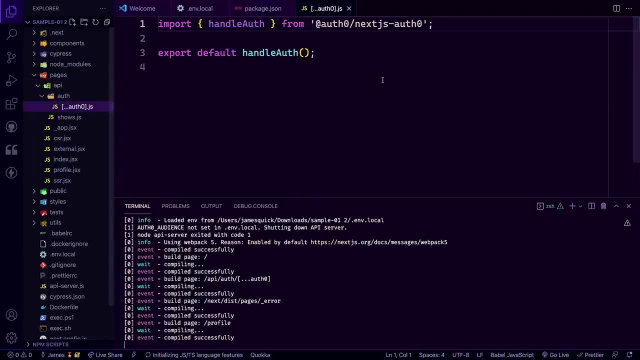 you will see that we have the Auth0, Nextjs, Auth0 package installed And then inside of our pages, directory, and then API and auth. you'll see we have a dynamic route here that exports this handle auth. Basically, this is all the configuration we need. 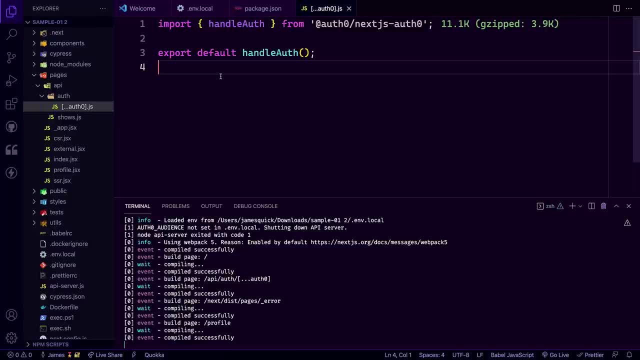 for the SDK itself to generate API endpoints for login, logout, callback and a me or a profile information route. So all of that stuff is configured for us. From there we can look inside of our components directory and inside of our navbar. 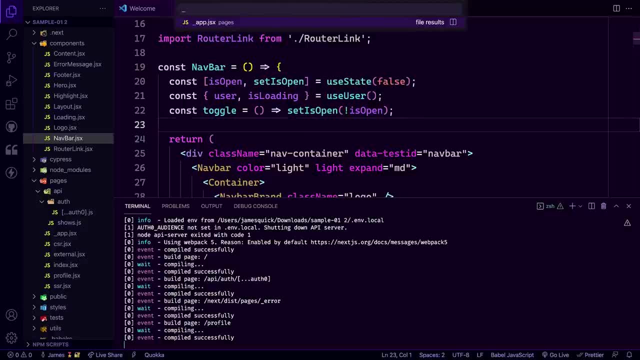 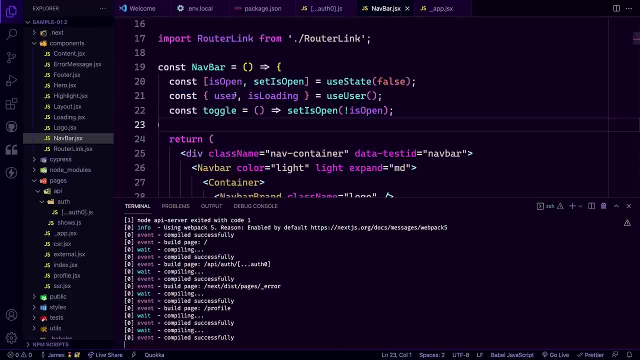 Notice there's a use user hook here. This is configured inside of the underscore appjs, where we wrap our entire app with the user provider, also provided by the SDK, And then we can access information about the user. We can determine whether or not they're logged in. 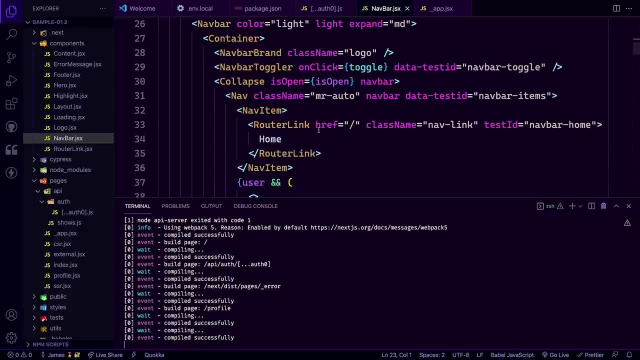 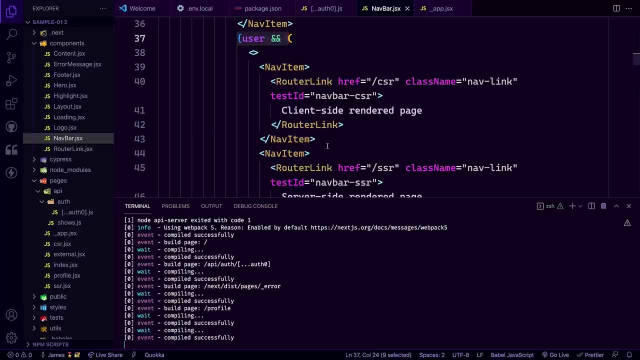 or if we're currently loading the user state and then show different things based on that. So you can see, here inside of our JSX, we're conditionally rendering a couple of different nav items based on if the user is logged in or not. 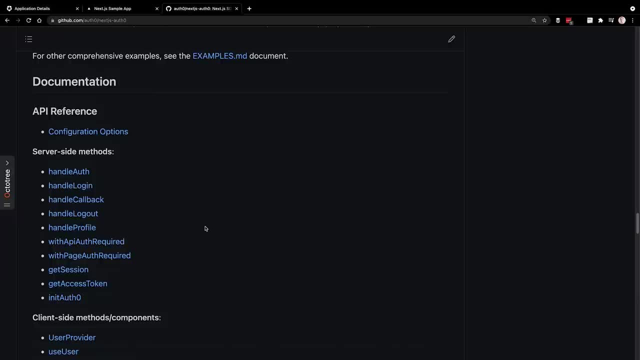 Now, if you're interested in a little bit more about what this SDK can do inside of Nextjs, you can check out the GitHub repository for all the details. A couple of things I want to call out are these higher order functions with API auth required.